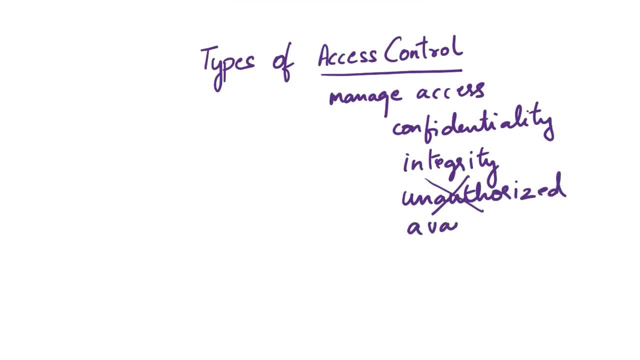 unauthorized access and to ensure availability of resources to authorized users. So, basically, access control aims to establish a secure and controlled environment by authenticating the users, that is, identify and authenticate the users and then authorizing their access based on their roles and permissions, and also maintaining accountability through 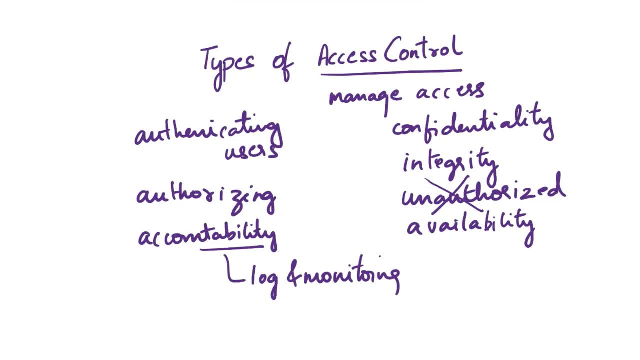 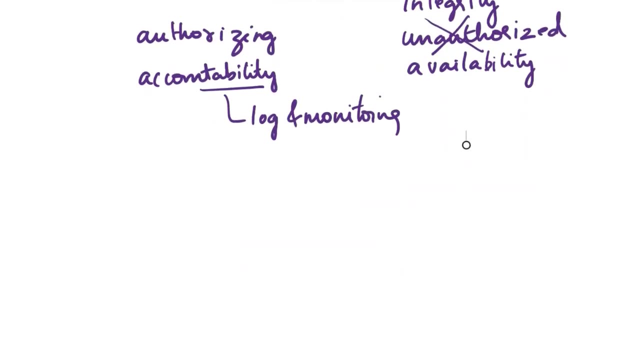 logging and monitoring. Now that we know what is an access control and what it aims at, what are its goals, Let's try to understand the different types of access control. Access control can be categorized based on how they are implemented or how what they do. Okay, first we'll see the types of access control based on how they are implemented. In this category, we have three types. First one is administrative access control. Next is technical or logical access control, and then we have physical access control. Administrative access control involves polices, procedures and measures implemented by administrators to manage access to resources and systems. Let's see some of the examples of administrative access control. The first one is access control policies. Here the administrators define and enforce access control policies that outline rules and guidelines for granting and managing access to. 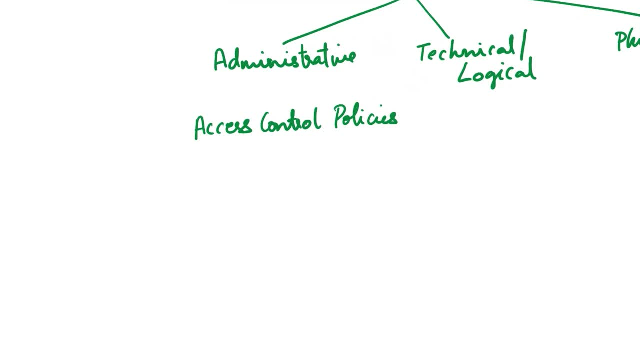 to resources. These policies specify who can access what resources, under what conditions and for what purpose. Next one is password policies. Administrators create these policies to ensure secure use of passwords. These policies may include requirements such as, you know, minimum password length, complexity, expiration periods, restrictions on password reuse, etc. Then we have 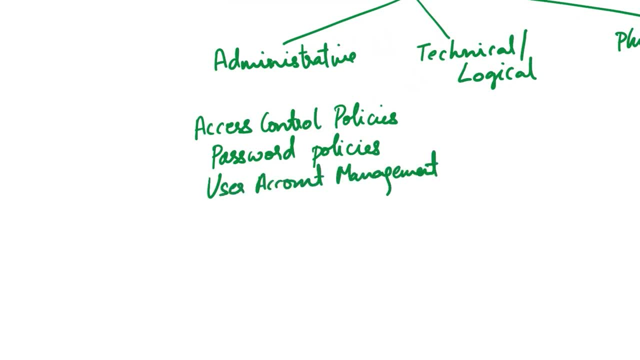 user account management. Administrators are responsible for creating, modifying and deleting user accounts. They control the process of granting and revoking access privileges based on user roles and responsibilities. Another example very close to this is user provisioning and deprovisioning. When an employee joins or leaves an organization, administrators are responsible for provisioning. 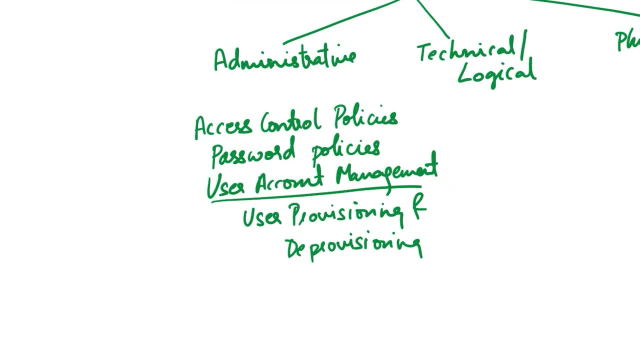 and deprovisioning user accounts. This is to ensure that access to the account is not limited to the user account. This is to ensure that access rights are granted promptly when needed and revoked when no longer that is required. Then we have the admins implementing RBAC. This is to 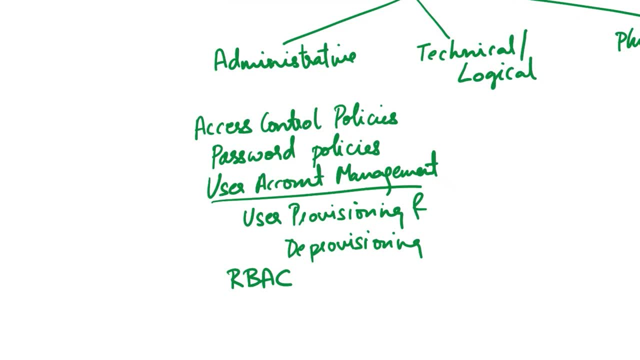 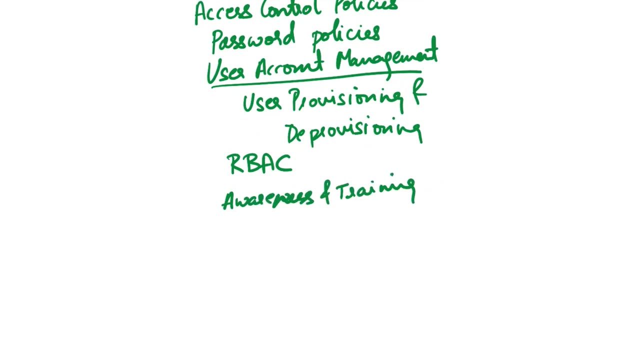 assign permissions to users based on their roles within the organizations. Roles define sets of permissions and users are assigned to appropriate roles based on their job functions. Then administrators also provide security awareness and training. This is to educate employees about control practices and the importance of maintaining security. This helps employees to understand their 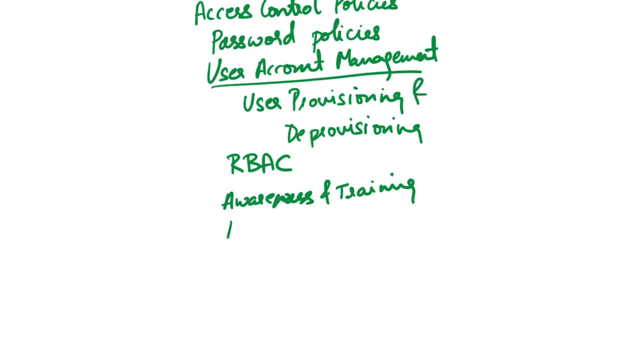 roles and responsibilities in safeguarding resources. Administrators also establish auditing and monitoring mechanisms. This is to track and log access activities. This allows them to detect and investigate any unauthorized access attempts or suspicious activities. So these are the examples of administrative access controls. Now let's see technical or 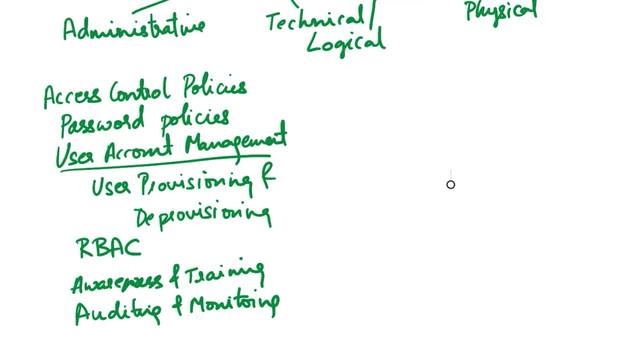 logical access control. Technical or logical access control refers to the use of technology, That is, the use of software-based, hardware-based or firmware-based measures to regulate and manage access to resources and systems. Let's see some of the examples of technical access control. 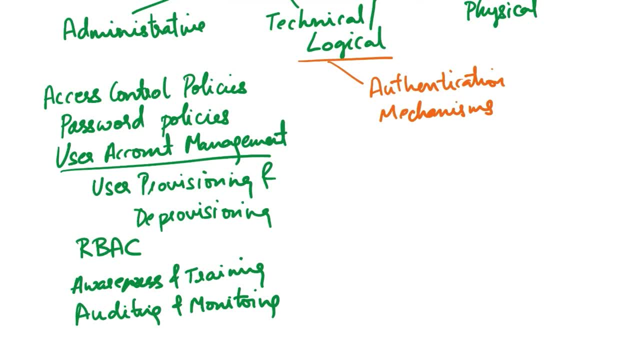 Authentication mechanisms like password-based authentication or biometric-based authentication, or you know you're using multi-factor authentication or two-factor authentication. That all comes under authentication mechanisms, under technical or logical access control. Another example is ACLs- access control lists. These lists are used to define and enforce. 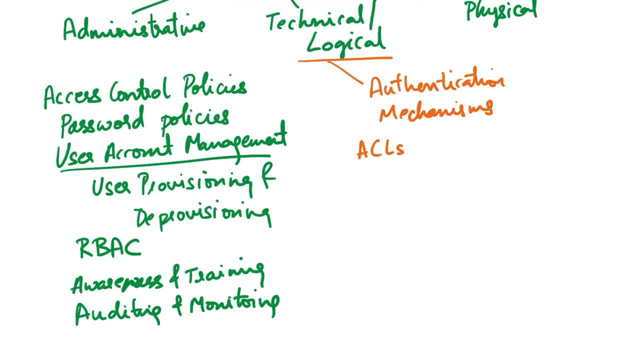 permissions on resources or systems. They specify who was allowed or denied access to specific resources based on user identities or groups. Another example is encryption. Encryption is used to protect data in transit and at rest. It ensures that only authorized individuals with the appropriate decryption keys can access and understand the data. Another example is: 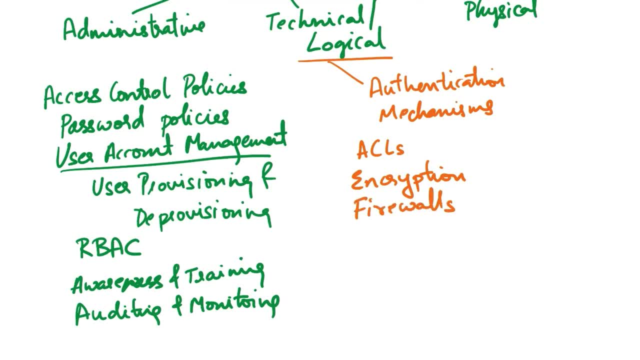 firewalls- Firewalls monitor and control incoming and outgoing network traffic based on predetermined rules. They protect systems and networks by filtering traffic and preventing unauthorized access. Another example is intrusion detection and prevention systems. PS monitors network or system activities for suspicious behavior or known attack patterns. 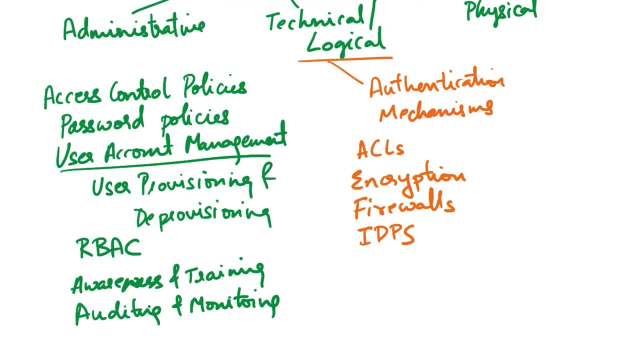 It can detect and prevent unauthorized access attempts or malicious activities. Another example is VPNs, that is, virtual private networks. VPNs establish secure connection over public networks, allowing users to access resources remotely while encrypting data transmission. Another example is SIEM, that is secure connection over public networks allowing users to access resources remotely while encrypting data transmission. 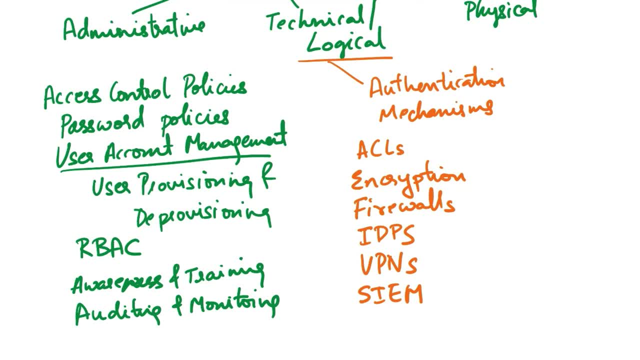 Another example is cybersecurity and security information and event management system. This collects and analyzes security event logs from various sources, such as access logs, to identify and respond to potential security incidents. So these are some of the examples of technical or logical access control. Now we'll see what is a physical access control. Physical access control involves 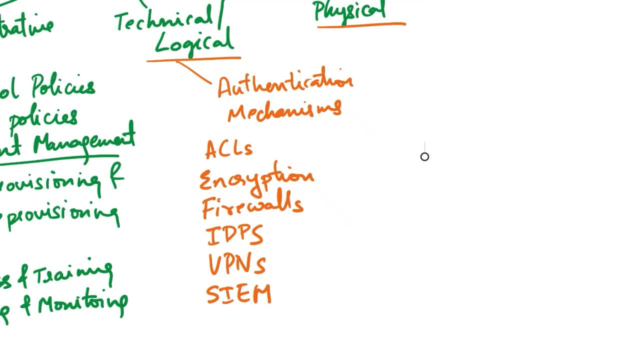 measures and mechanisms to regulate and manage physical access to buildings, facilities or within an organization. let's see some of the examples. the first one is physical barriers. these are used to restrict access to specific areas like, for example, fences and gates. turnstile turnstiles allow only one person to pass through at a time, ensuring controlled access. okay, and then? 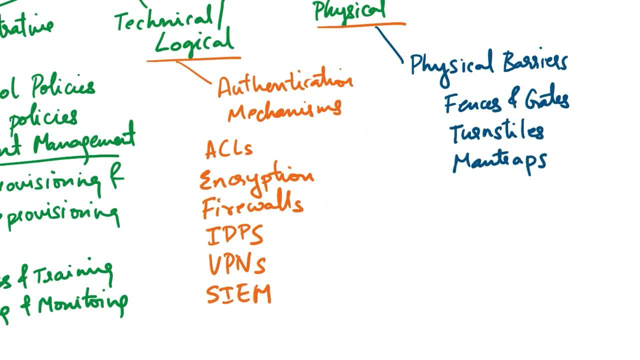 we have man traps. a man trap is an enclosed space with two doors where one door must close before the other opens, allowing only one person at a time. these are the physical barriers. then we have locks and keys. traditional locks and keys are commonly used to secure doors and restrict access. 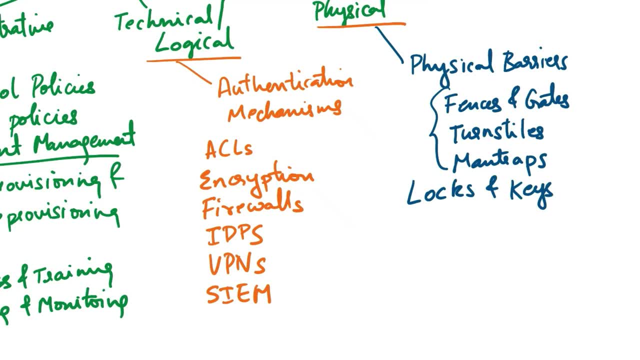 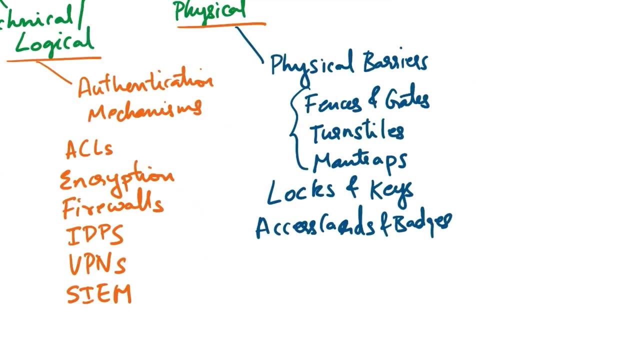 to authorized personnel only. different types of locks, such as padlocks, deadbolts or electronic locks, can be employed, based on the level of security that is required. another example is access cards and badges. these are issued to authorized individuals and are used to gain entry through card readers or electronic access control systems. these cards can be: 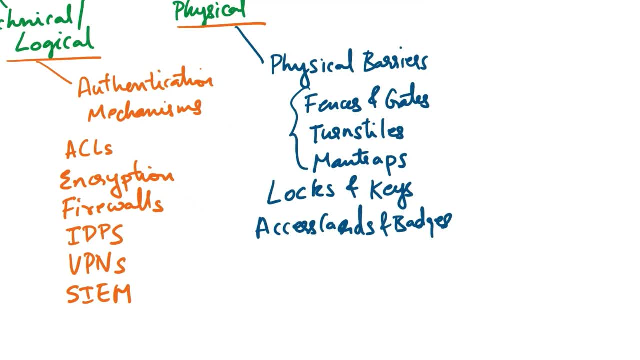 programmed to grant specific access privileges to different areas or zones. and then we have biometric systems. this utilizes unique physical characteristics of individuals for identification and authentication, like, for example, fingerprint scanners, retina or iris scans or even facial recognition. and then we have a surveillance systems, like, for example, surveillance cameras, are used to monitor and record activities. 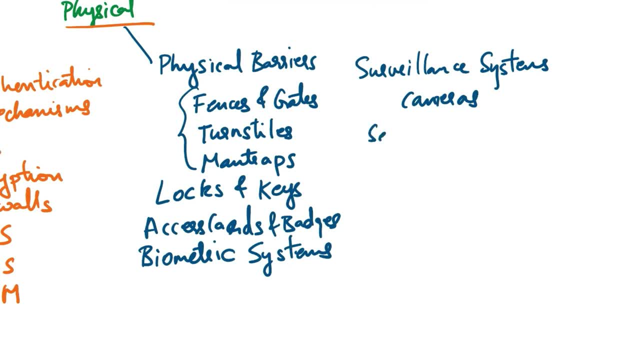 in and around the facilities. then security guards. security guards are stationed at entry points or designated areas to ensure only authorized individuals gain access and to respond to security incidents. then we have visitor management systems. these systems track and manage visitors access to facilities. they typically involve registering visitors to the facilities and 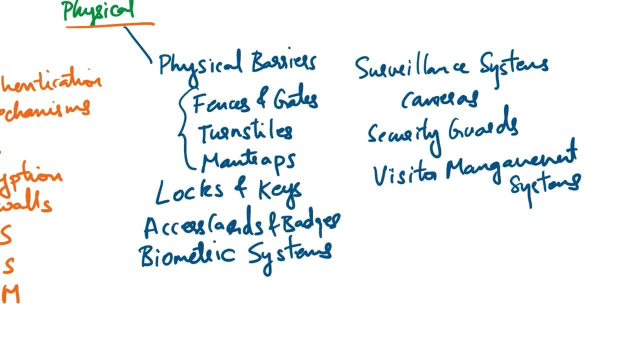 visitors, issuing visitor badges and monitoring their activities during their visit. then we have alarm systems. this includes motion detectors or intrusion detection sensors. these are used to detect unauthorized access attempts and trigger an alarm or alert security personnel. then there is physical access locks. recording and maintaining logs of physical access activities provide an 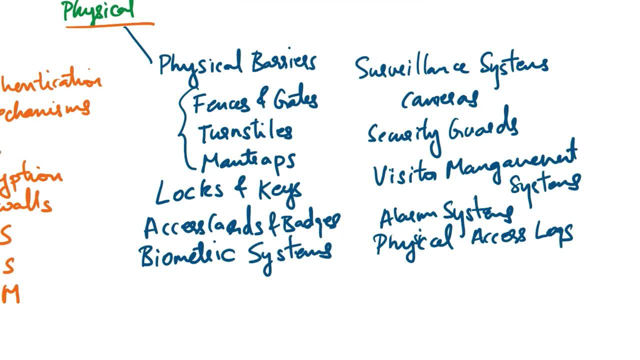 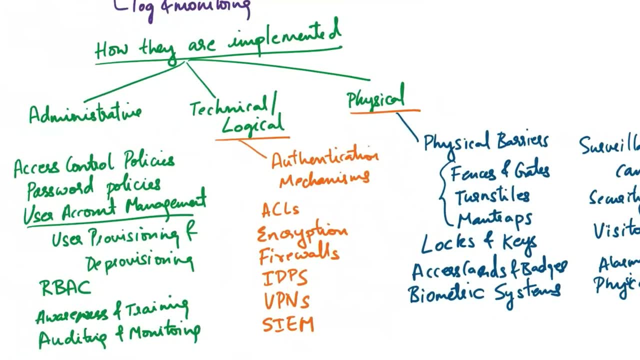 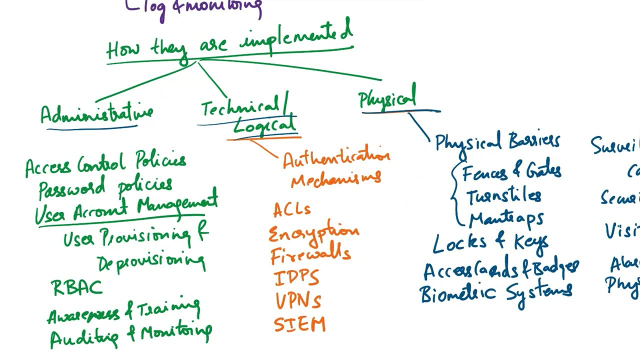 audit trail and help monitor and investigate any security incidents or activities that are happening in the area. so these are the examples of physical access control. now we know the category based on how they are implemented, that is, administrative, technical or logical and physical access controls. now we'll move on to the types of access control that are categorized based on. 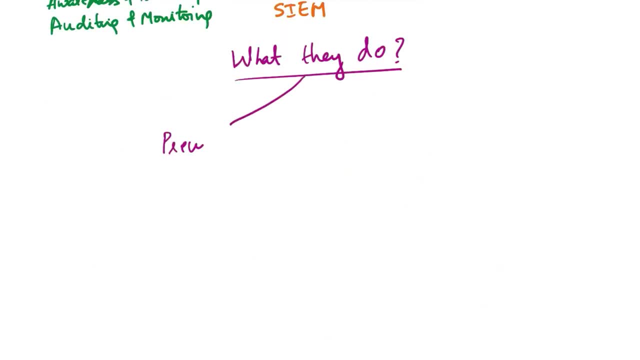 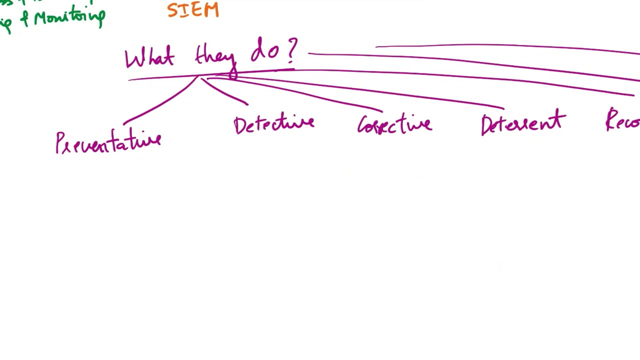 what they do. in this we have first one we'll talk about as preventative access control or preventive access control, then there is detective, then corrective access control, then deterrent access control, then we have recovery access control, then there is directive access control and then compensating access control. preventive access control refers: 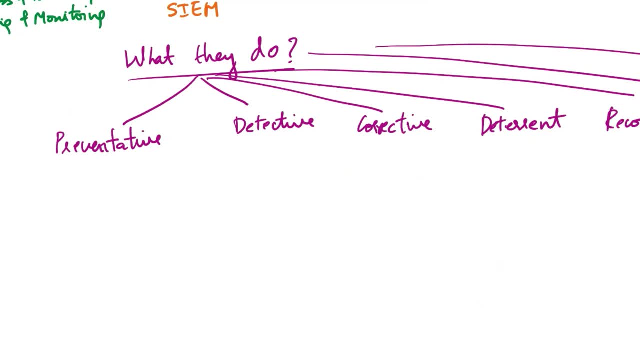 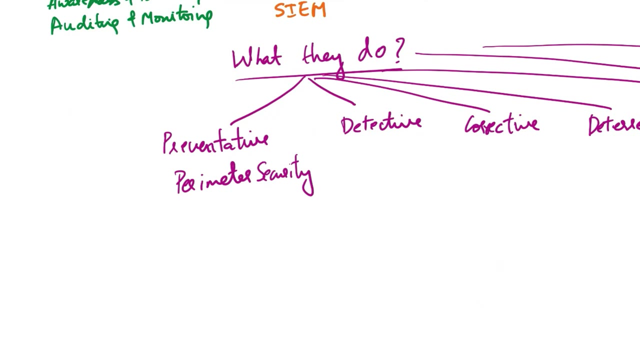 to the measures and strategies implemented proactively to prevent unauthorized access and potential security breaches, like, for example, perimeter security: physical barriers such as fences, walls, gates installed to secure the perimeter of a facility or property. this prevents unauthorized individuals from easily gaining access to the premises. then security signs, like you know, visible signs. 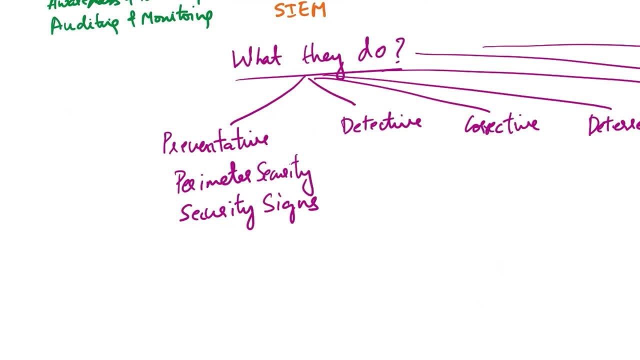 indicating restricted areas, video surveillance, alarms or warning messages also prevent access. also, access control systems like implementing electronic access control systems helps prevent unauthorized access to buildings or specific areas within a facility. like you know, you're using card readers, keypads, biometric systems that require authorized credentials for entry. 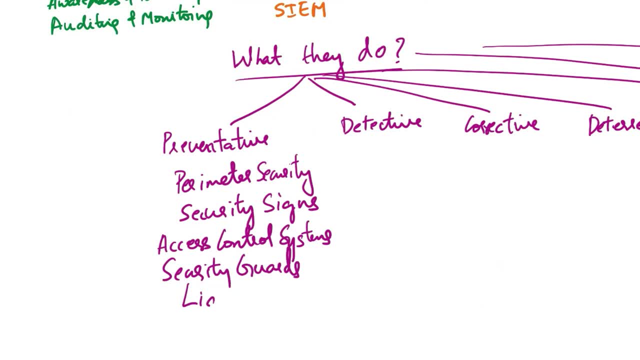 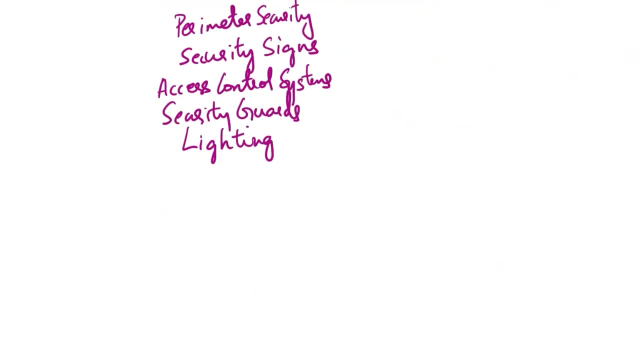 then security guards also. proper lighting, like lighting in and around the premises, reduces the likelihood of unauthorized access by making it difficult for individuals to go unnoticed. you can also use motion activated lights, then installing camera us then having firewalls, intrusion detection and prevention systems, antivirus software, security. 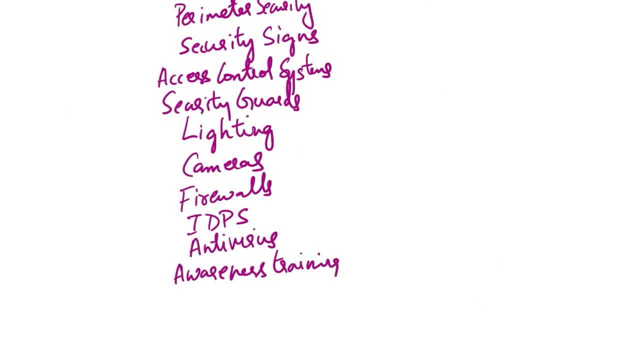 awareness training here, educating employees and users about security best practices, policies, procedures- raises awareness and helps prevent social engineering attacks, unauthorized sharing of credentials or negligent behavior that could compromise access control. then security policies and procedures. establishing comprehensive security policies and procedures ensures that access control measures are consistently followed and enforced across the organization. this includes defining strong 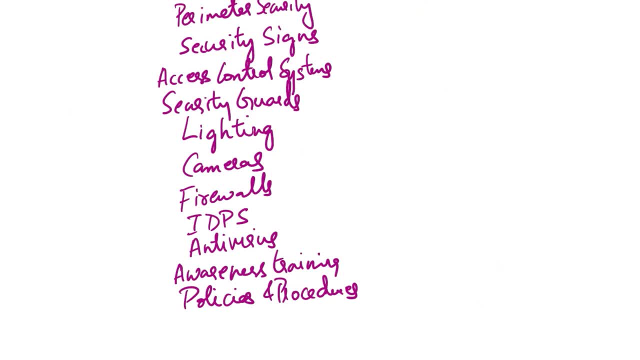 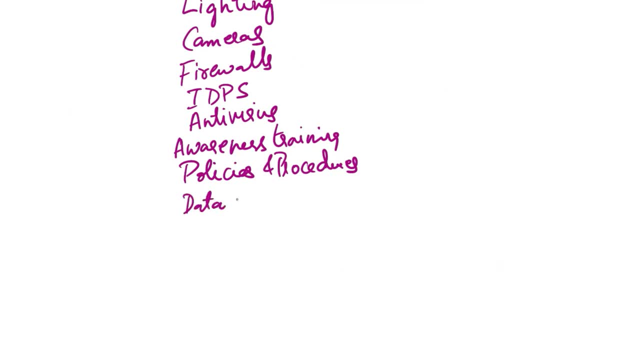 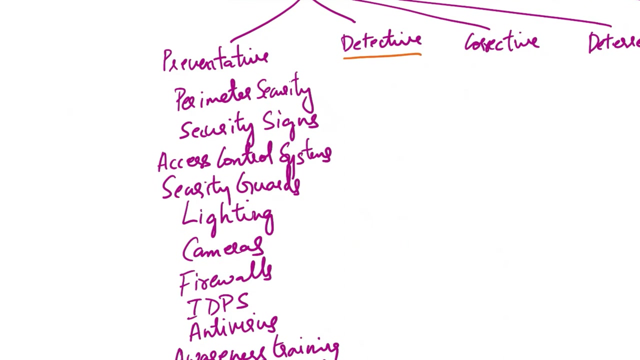 password policies, access revocation processes, incident response procedures and so on. and the other examples of preventative access control is data classification, penetration testing, job rotation policies, separation of duties policies and the other examples of preventative access control. so the list goes on. okay, that is about preventative access control. then we have detective access control. 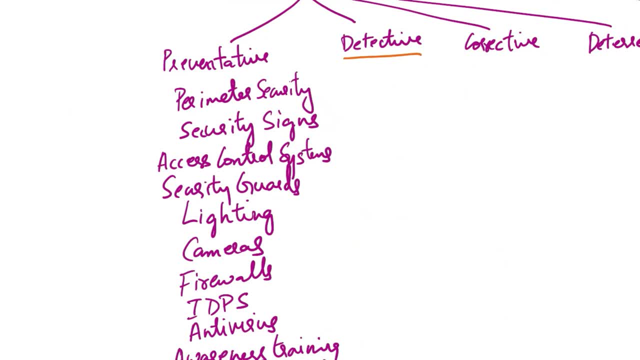 this refers to measures and strategies implemented to detect and identify unauthorized access or security breaches after they have occurred. okay, these controls focus on monitoring and analyzing activities to identify anomalies or suspicious behavior. let's see some of the examples of detective access control, security logging and auditing and monitoring of activities to identify. 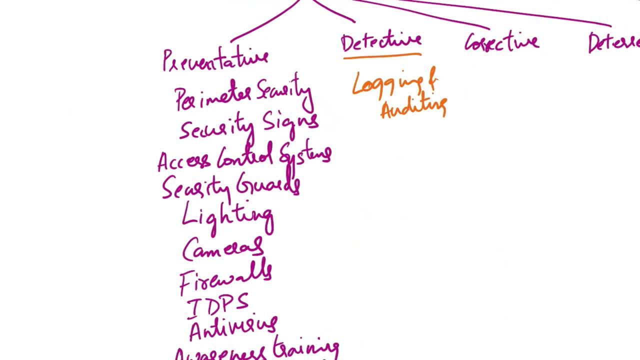 unauthorized access or suspicious behavior. and auditing. implementing robust logging mechanisms to record access events, system activities and user actions and then reviewing these logs regularly or analyzing to detect. analyzing these logs to detect unauthorized access attempts or suspicious activities can implement detective access control. then we have a sim: security information and event. 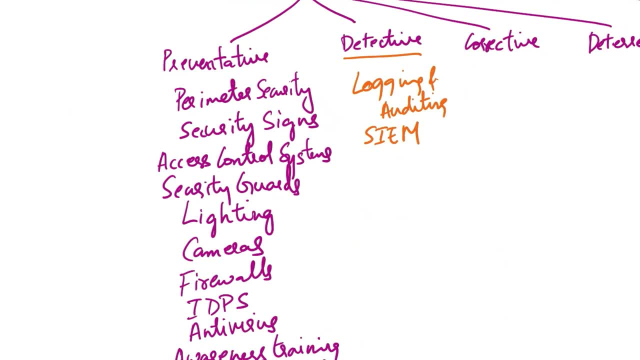 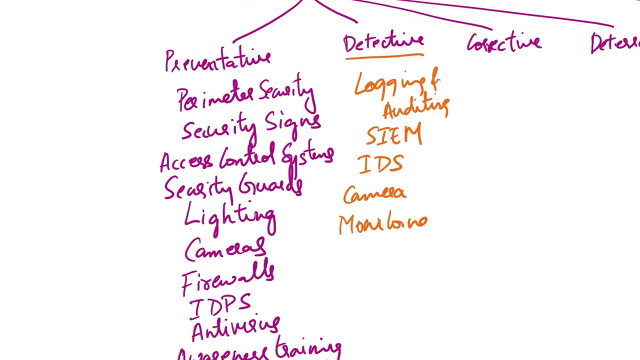 management system that collects and correlates security logs from the system to the system and from various sources. then there is intrusion detection systems and then cameras and video surveillance. then there is monitoring tools system and network monitoring tools. then we have uba- user behavior analysis. uba solutions analyze user behavior patterns and 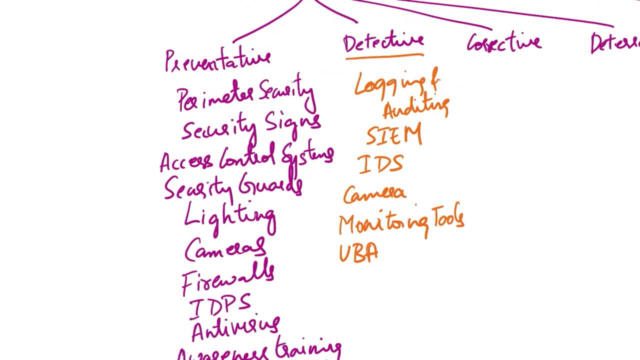 baseline normal behavior. okay, then they can detect anomalies such as unusual login times, access to unauthorized resources or excessive data downloads which may indicate unauthorized access or compromised accounts. then incident response planning. having an incident response plan in place allows organizations to quickly detect and respond to security incidents. it includes procedures for detecting and. 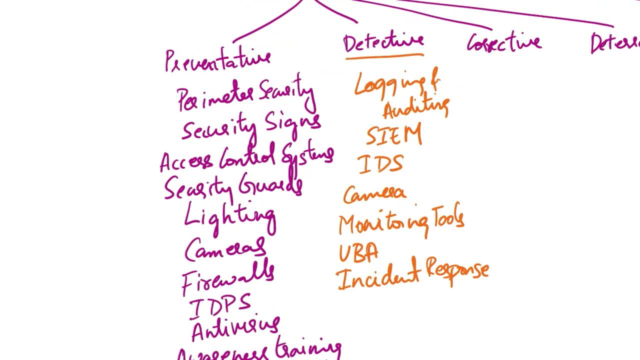 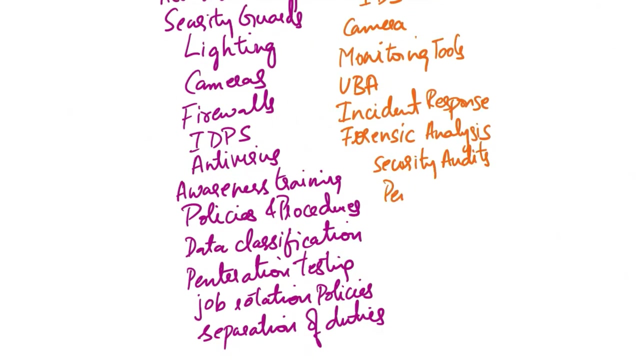 investigating unauthorized access, containing and mitigating the impact and restoring normal operations. then we have forensics analysis. these are the techniques that are employed to examine digital evidence, such as access logs, system snapshots or network captures, to reconstruct the sequence of events and determine the extent of the breach, then security audits and pen tests, that is, 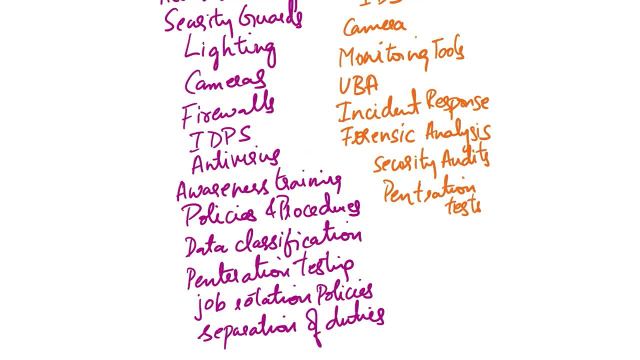 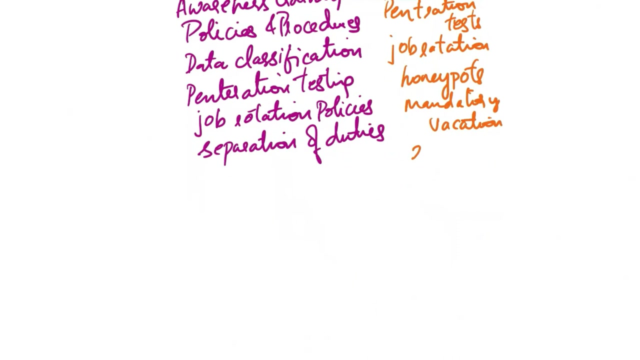 penetration tests can help identify vulnerabilities or weaknesses in access control systems. these activities aim to detect potential security gaps before they are exploited by unauthorized individuals. then job rotation policies and also you know you can install honeypods or honeynets to identify, detects any compromise. then you know you can have mandatory vacation policies. then there can be reviews of. 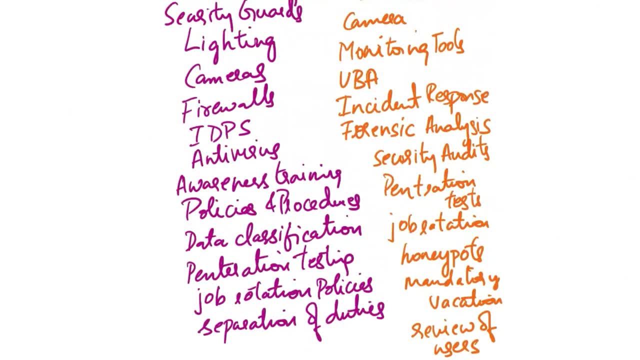 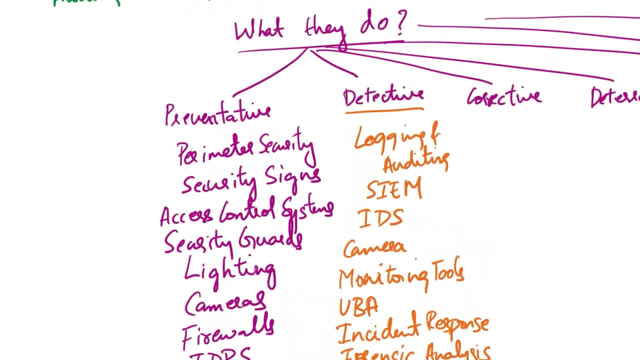 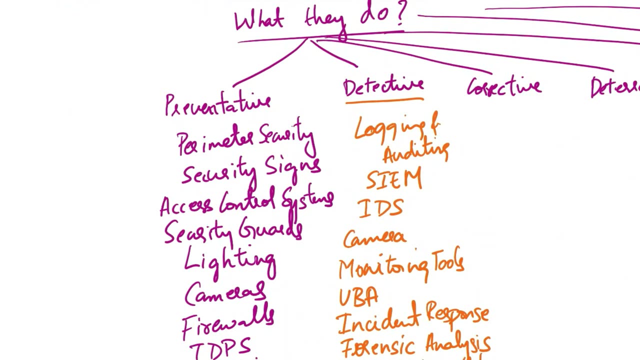 the users and their accesses. so if you notice here, right, many of the examples fall under many categories, like job rotation policies can be a preventative access control as well as a detective control. it doesn't like it doesn't have to fit in one type. it can fall under many types, like 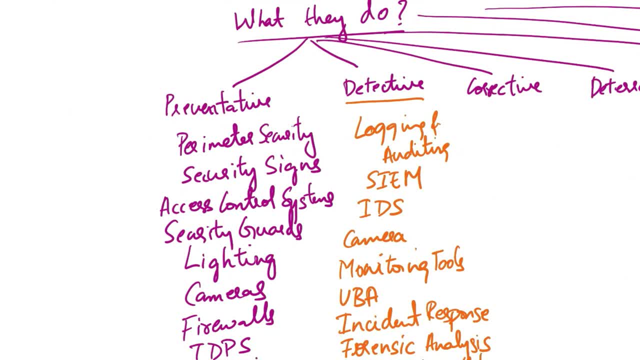 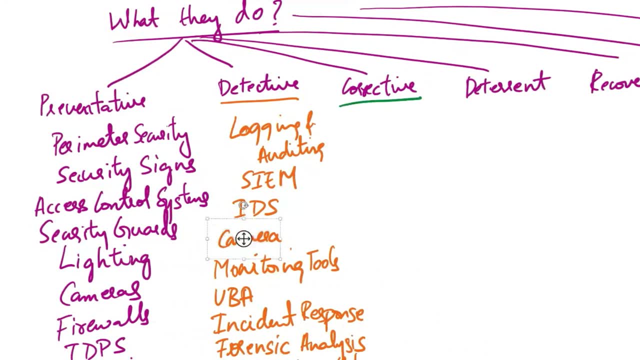 security cards. they can detect a malicious activity. also, they can prevent a malicious activity by intervening. next one is corrective access controls. this refers to measures and actions taken after an unauthorized access or security breach has been detected. the purpose of corrective controls is to mitigate the impact of the incident. 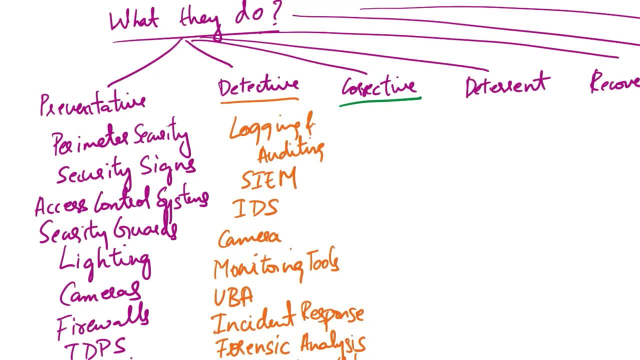 restore security and prevent future occurrences. let's see some of the examples. the first one is incident response and management. establishing a formal incident response plan that outlines the steps to be taken when a security incident occurs is very important. this includes identifying the incident, containing the impact and conducting the investigation and implementing remediation plans. 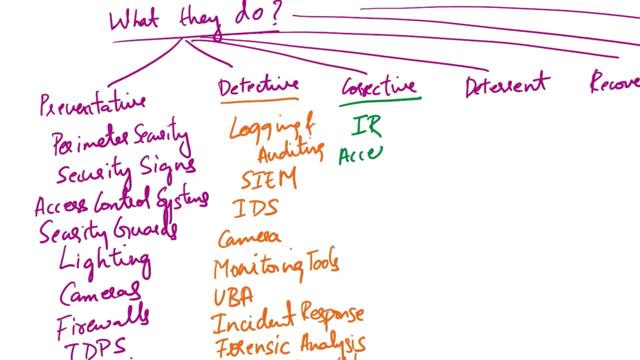 remediation measures. then there is access revocation: disabling or revoking access privileges of compromised accounts or individuals involved in an unauthorized access. this ensures that unauthorized users no longer have access to resources and systems. then there is system patches and updates. applying security patches, updates or fixes to address vulnerabilities that are exploited during the unauthorized access is to. 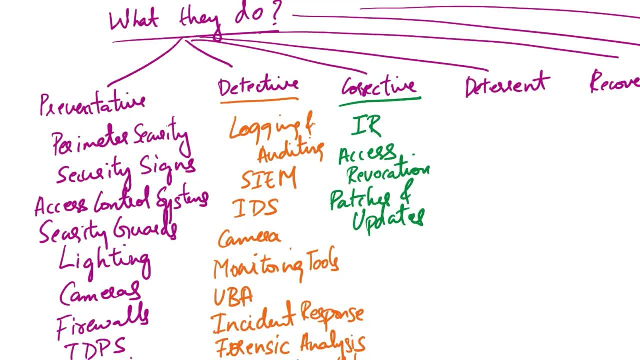 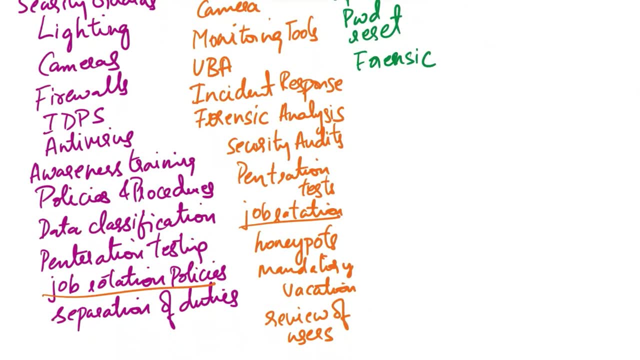 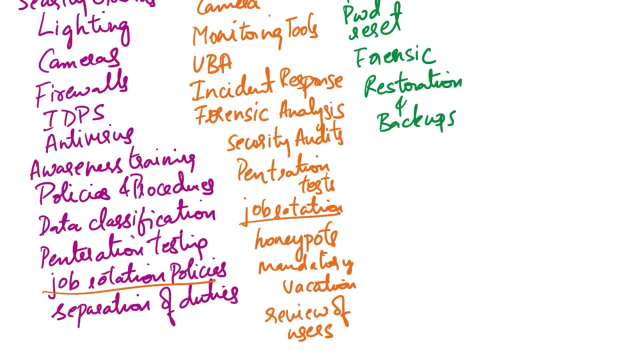 help prevent similar incidents from occurring and to prevent similar incidents from occurring in the future. then there is password reset, forensic analysis. then we have a system restoration and backups. that does, restoring affected systems to known secure state using backups or system snapshots. this helps eliminate any malicious changes made during the unauthorized access and 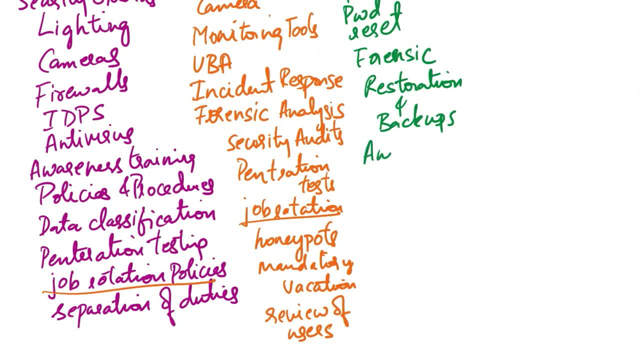 ensure systems are free from compromise, security awareness and training, providing additional security awareness training and security awareness training and security awareness training to employees and users. here we focus on the lessons learned from the incident. this helps enforce security practices, educate users about the potential threats and enhance their vigilance. 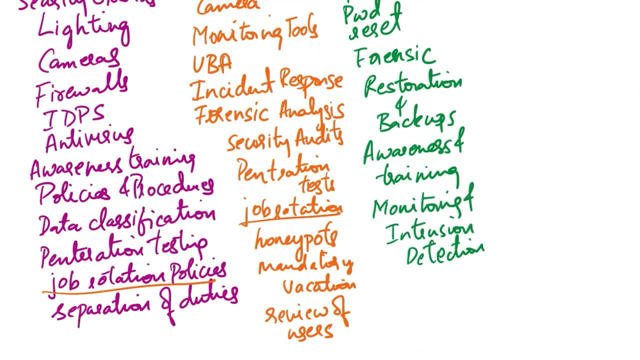 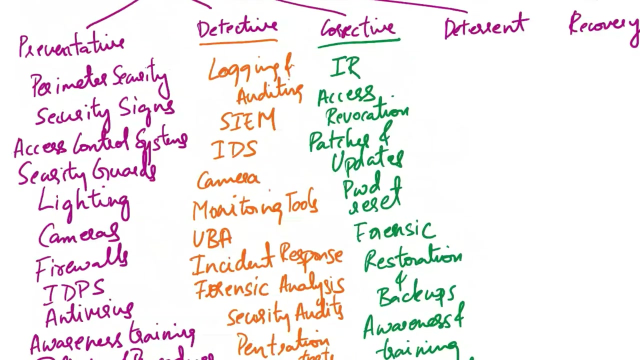 continuous monitoring and intrusion detections. strengthening monitoring systems and intrusion detection mechanisms will can help to detect and respond to similar unauthorized access attempts or security breaches, and real-time systems that can help to prevent or, you know, remove or quarantine a virus or a malware. so all these are examples of corrective access control. then we have deterrent access control. 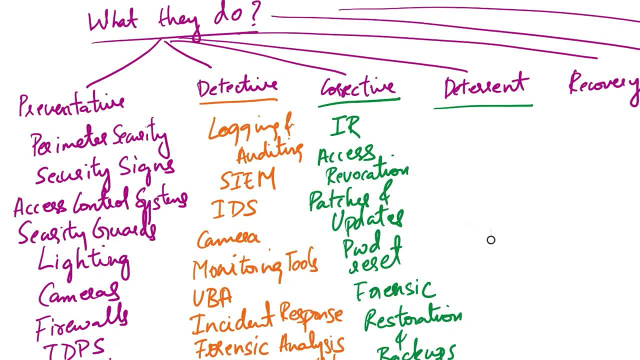 deterrent access control refers to measures and strategies implemented to discourage potential unauthorized access or security breaches by creating a perception of risk or increasing the effort required to breach security measures. this is to discourage- okay, the goal is to deter potential intruders from attempting unauthorized access. examples include visible security measures. 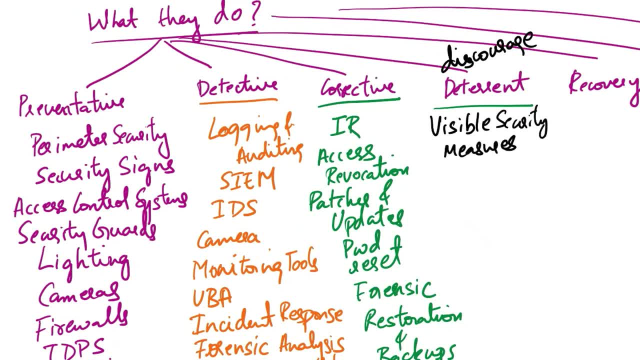 like surveillance cameras, access control systems or security guards can create a sense of being monitored and increase the perceived risk of detection. we can also have warning signs and labels, that is, to place warning signs, labels or notices indicating that the area is under surveillance, restricted or protected by security measures. these signs act as a psychological deterrent. 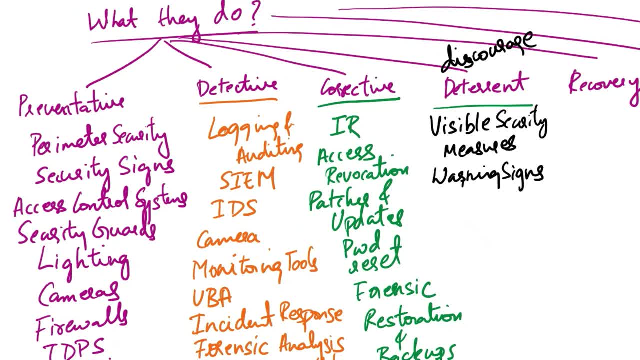 by making potential intruders aware of the consequences of unauthorized access. then fencing and barriers: installing physical barriers, fences or gates around the premises to clearly define the boundaries and demonstrate a control and control of the area. and the area is under surveillance, restricted or protected. and the area is under surveillance, restricted or protected. 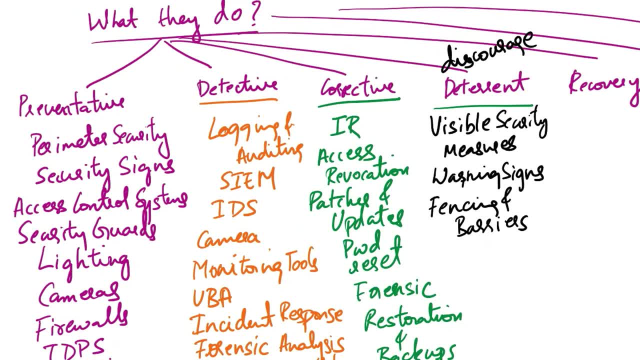 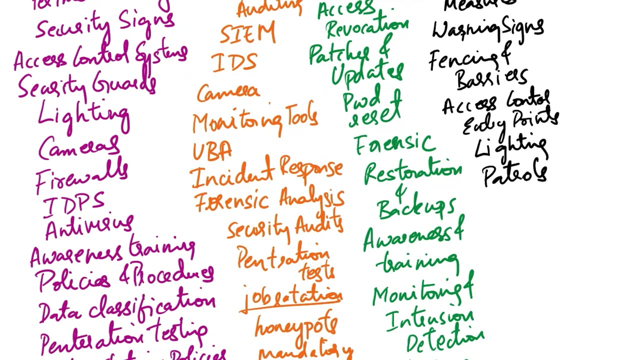 environment can also help deterring the access. then access control: entry points. the presence of these control mechanisms acts as a deterrent, signaling that only authorized individuals are allowed entry. then you know lighting adequate lighting in and around the premises. then security patrols. these are regularly conducted by security personnel or guards and these can help deter. 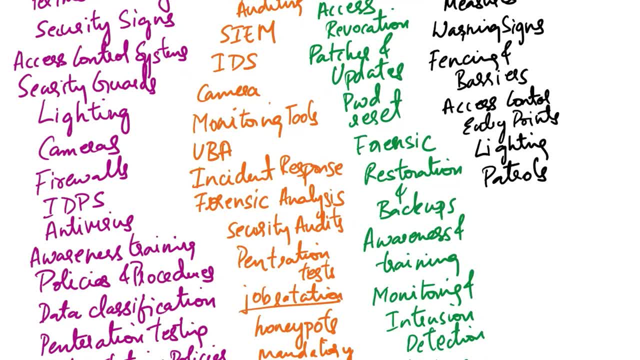 unauthorized access by providing a sense of security and a sense of security. and a sense of security can also help deter the presence of a person at the premises, so that this one that's what's happening. the security equipment is that is used to detect the presence of a person. 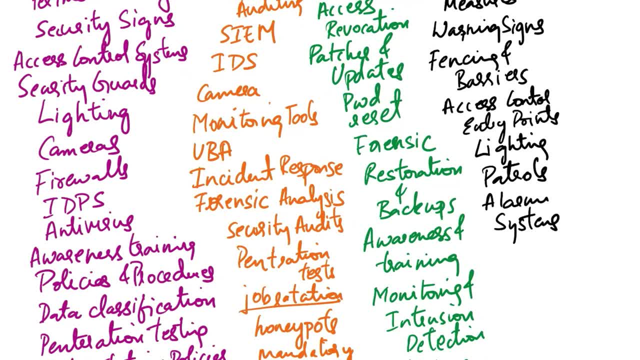 then alarm systems. like you know, installing audible alarm systems that activate when unauthorized access is detected can serve as a strong deterrent. then secure storage and equipment. securely storing valuable assets or equipment in locked cabinets, safes or, you know, secure rooms with restricted access can also act as a deterrent. then awareness of the presence of a person on a particular site. 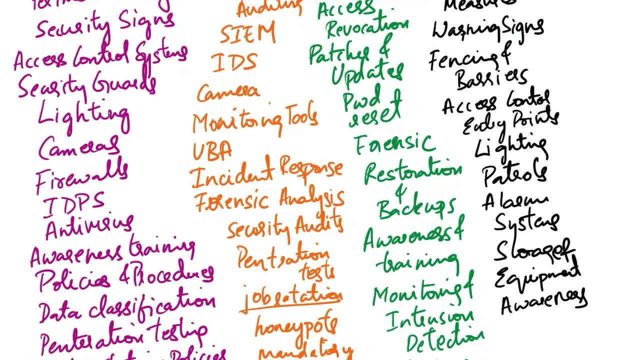 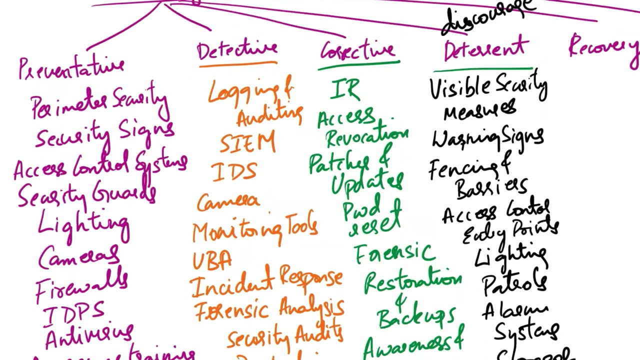 programs, implementing security awareness programs that educate employees and users about the importance of security measures, proper access control procedures and potential consequences of unauthorized access can create a culture of vigilance and enforce the message that security is taken seriously. so these are the examples of deterrent access control. then we have recovery access control. recovery access control refers to measures and: 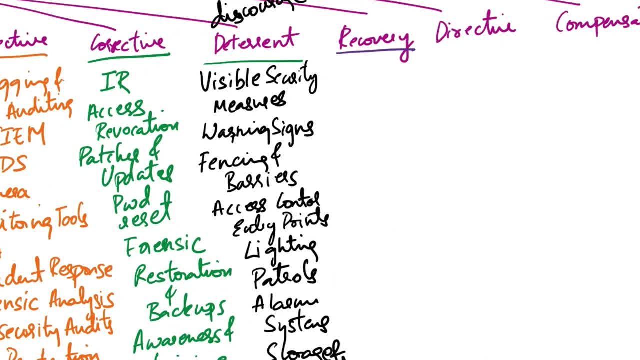 actions taken to restore normal operations, mitigate the impact of a security incident and recover from the consequences of unauthorized access or security breaches. the focus is on recovering from the incident and minimizing downtime or damage. let's see some of the examples of recovery access control. the first one is incident response. 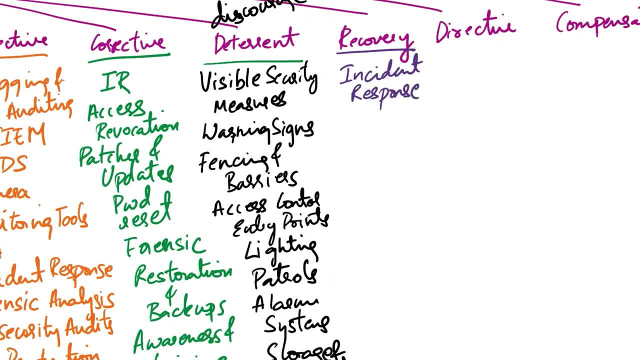 response plan execution. so, following the incident response plan, which outlines these steps to be taken during and after a security incident, can act as a recovery access control. this includes assigning responsibilities, coordinating actions and executing the plan to ensure a structured and efficient recovery process, also documenting the details of the incident, including its impact. 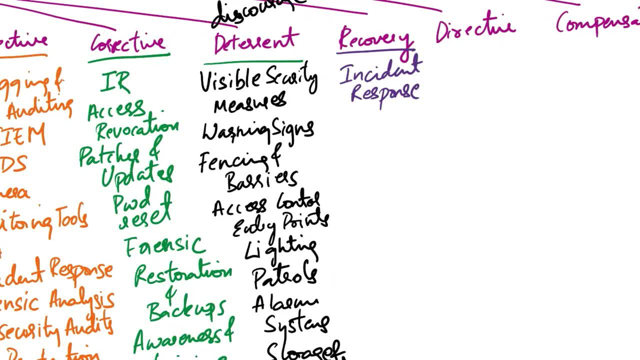 root cause analysis and the actions taken for recovery helps to ensure a secure and efficient recovery process in post-incident analysis, identifying areas for improvement and implementing preventive measures. another example is system restoration: restoring affected systems, applications or data to a known secure state using backups or recovery mechanisms. implementing change management procedures to review and validate system changes before they are implemented. this helps prevent similar incidents in the future and ensure that any changes made during recovery are thoroughly assessed and authorized. then we have patch management, applying security patches, updates or fixes to address vulnerabilities that were exploited during the unauthorized access. this helps prevent the same. 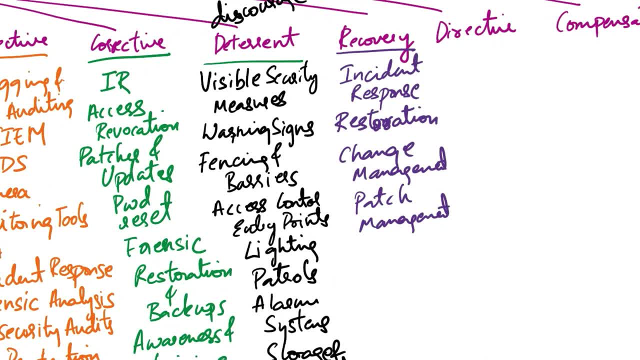 vulnerabilities from being exploited in the future and enhances system security. then there is user account remediation: reviewing and updating user accounts to revoke access privileges of compromised or unauthorized accounts ensures that only authorized individuals have access to the systems and resources. then then system hardening: strengthening security configurations, tightening access controls and 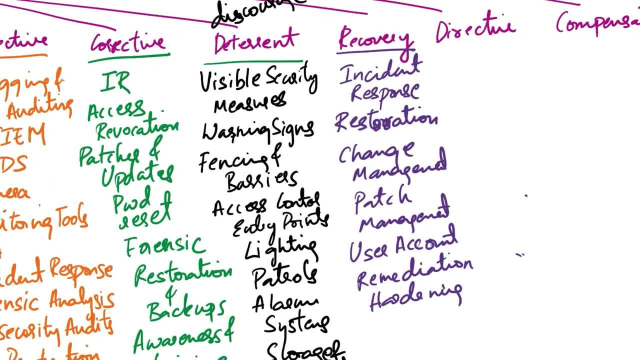 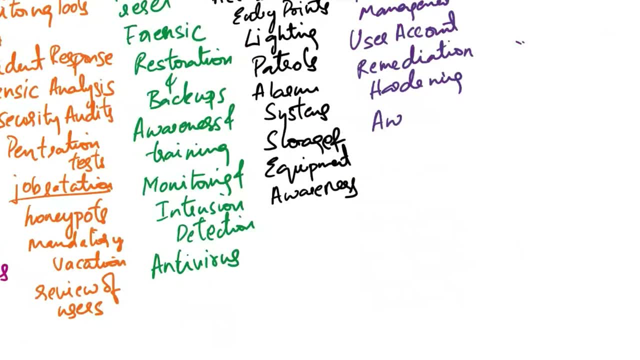 implementing security best practices to ensure the security posture of systems and prevent future unauthorized access. then there is security awareness training. this is to educate employees and users about the incident, its impact and measures, and then lessons learned and continuous improvement. we should conduct a post incident review to identify lessons learned gaps. 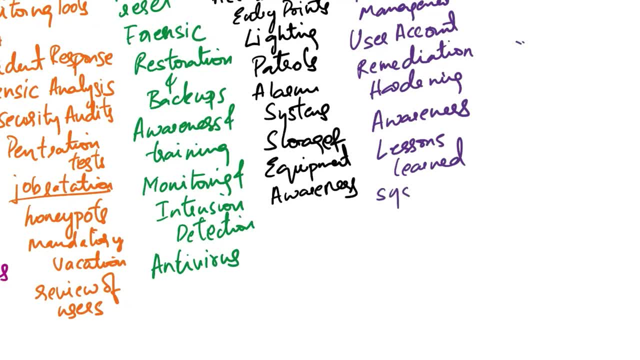 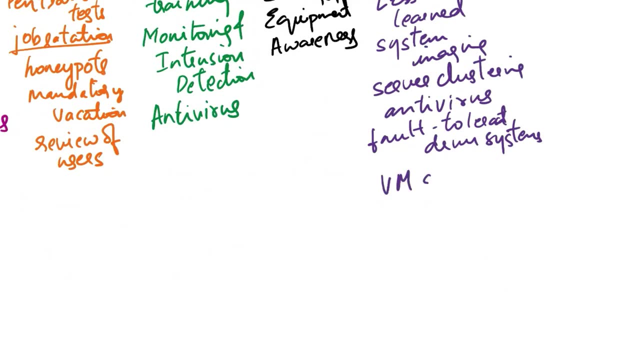 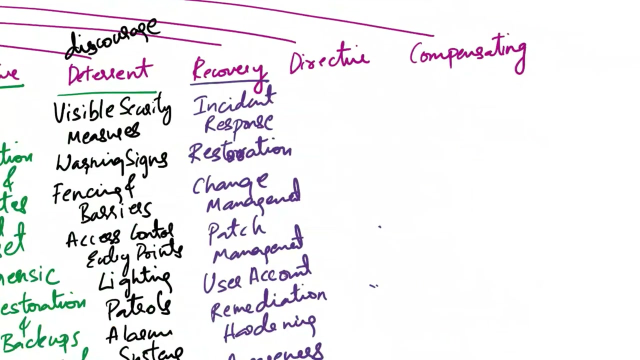 in security controls or areas for improvement. other examples are system imaging, server clustering, having an anti-virus or anti-malware solution, fault tolerant drive systems, virtual machine shadowing or database shadowing. so these are the examples of recovery access control. then we have directive access control. directive access control is where you direct or try to tell the subjects or 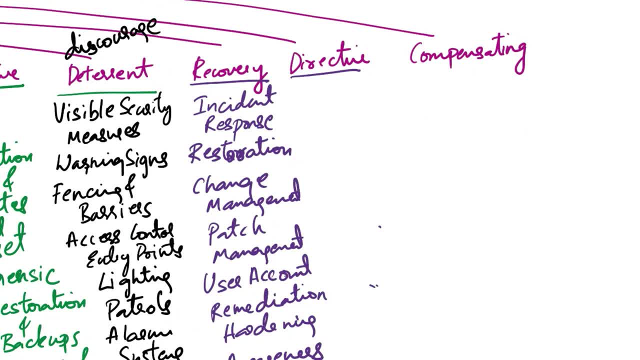 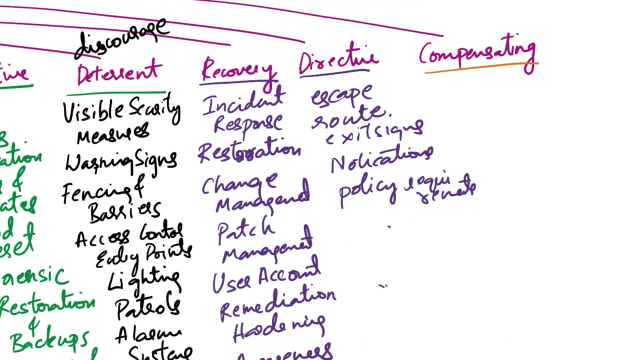 to control the actions of the subjects to enforce or encourage compliance with security policies, like, for example, escape route exist, exit signs, notifications, security policy requirements, etc. then there is compensating access control. compensating access control refers to supplementary measures implemented to address vulnerabilities or deficiencies in primary access. 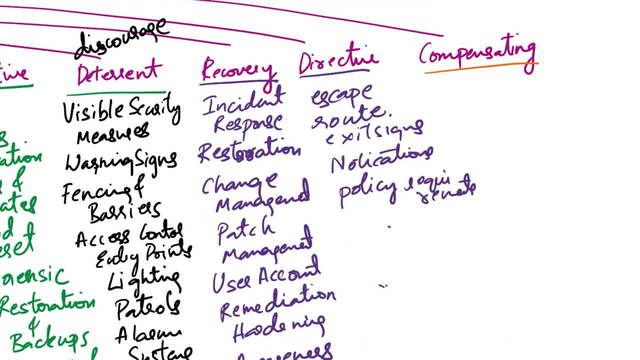 control mechanisms. these compensating access controls are put in place when acts primary access controls are not feasible, practical or sufficient to adequately mitigate risks. they help to compensate for the limiting or gaps in the primary controls and enhance the overall security posture. let's see some of the 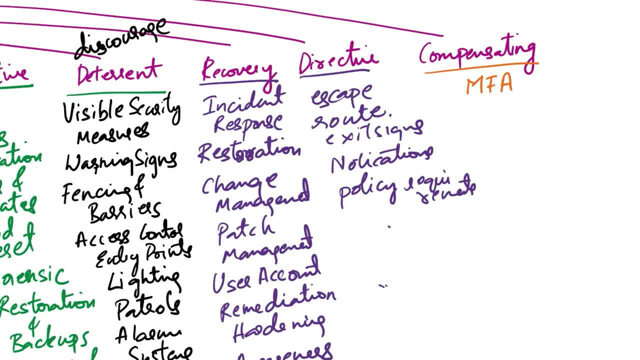 examples. first one is multi-factor authentication, implementing mfa as a compensating control when strong password policies alone may not provide sufficient protection. mfa requires users to provide multiple forms of authentication, such as a password and a one-time passcode sent to their mobile device, adding an extra layer of authentication to the security posture. 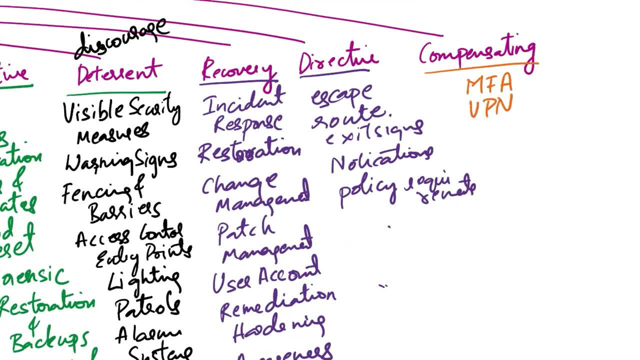 to stop communication management and to ensure safe and secure security. then using vpns, that is, virtual private networks as compensating controls can secure remote access to networks or sensitive systems. vpns establish encrypted connections over public networks, providing secure access to resources and compensating for the inherent risks of remote connectivity. then data: 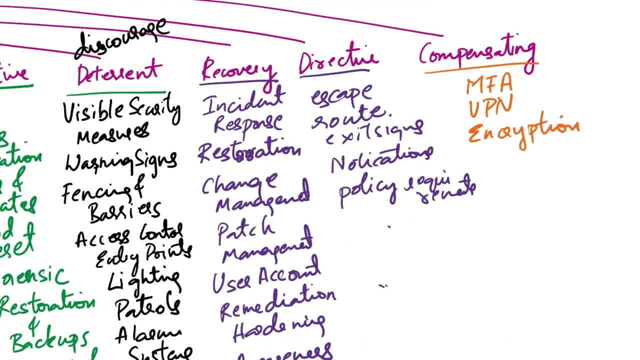 encryption, that is, to apply encryption to sensitive data at rest and ensure risk reduction and transit. encryption compensates for vulnerabilities in storage systems or communication channels, ensuring that even if unauthorized access occurs, the data remains unreadable and protected. then a sim solution: security information and event management system. this can be used as a compensating. 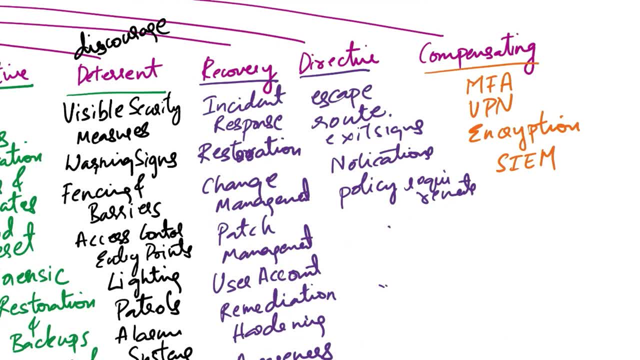 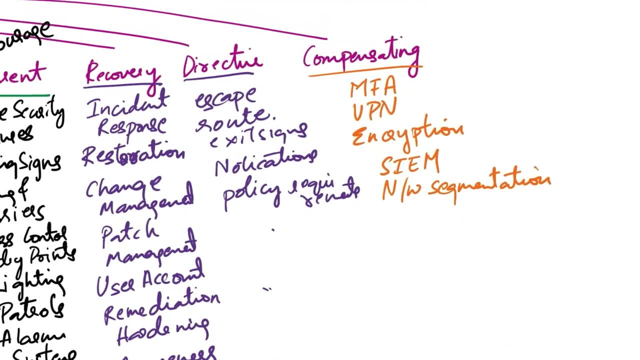 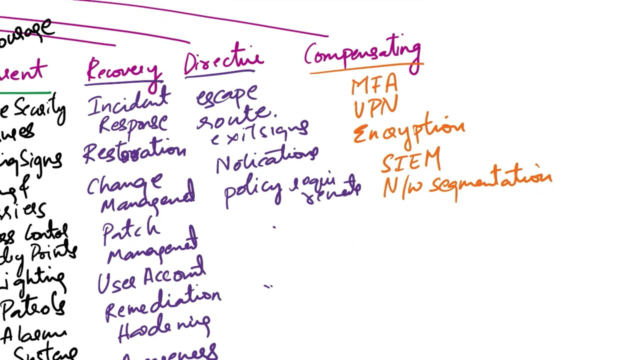 control to monitor and analyze logs from various systems and applications, and it enhances the ability to detect and respond to security incidents by aggregating and collecting the event data. also, network segmentation: implementing network segmentation to isolate sensitive systems or data from the rest of the network can limit the impact of the security of a security breach. 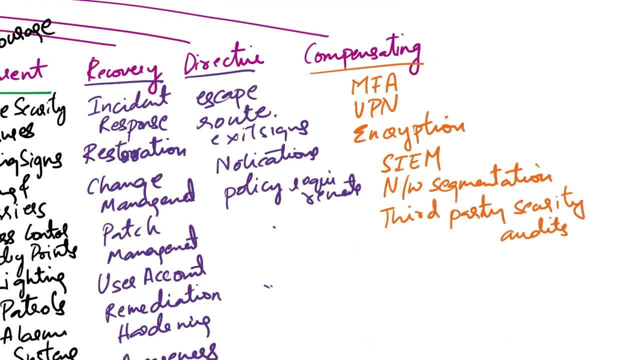 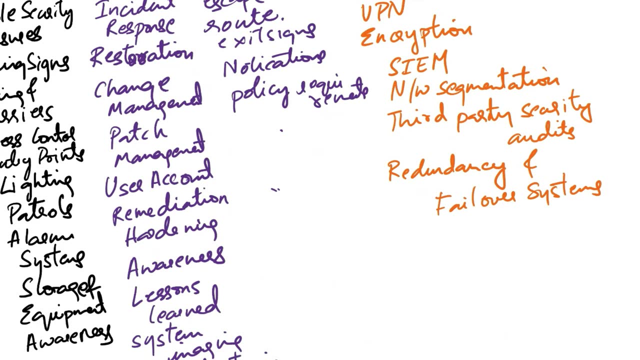 then third-party security audits: conducting third-party security audits and assessments to identify vulnerabilities and ensure that compensating conducts security audits and assessments to identify vulnerabilities and ensure that controls are effectively implemented. then redundancy and failover system. this compensates for potential system failures or outages. redundancy ensures that if one system or 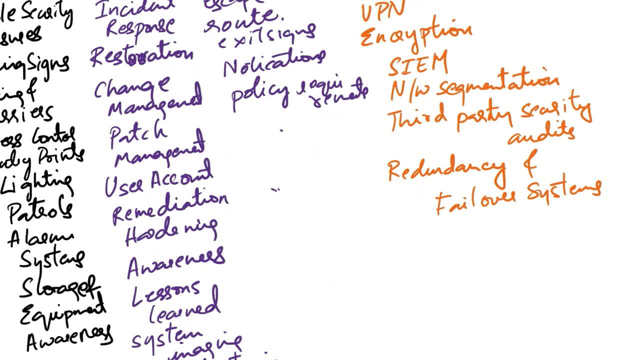 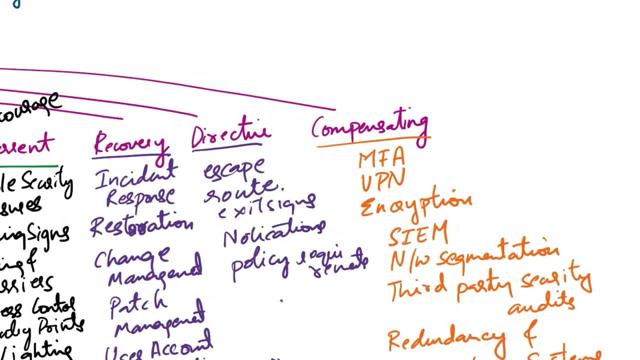 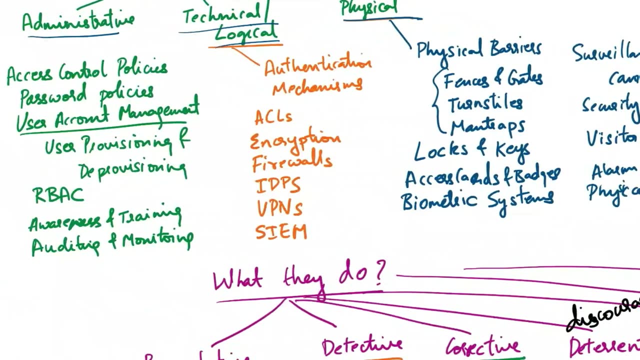 component fails, the backup systems can seamlessly take over, minimizing disruption and unauthorized access opportunities. so these are some of the examples of compensating access control. so now you should be able to answer: what is an access control? the goal of access control is to ensure that only authorized individuals have 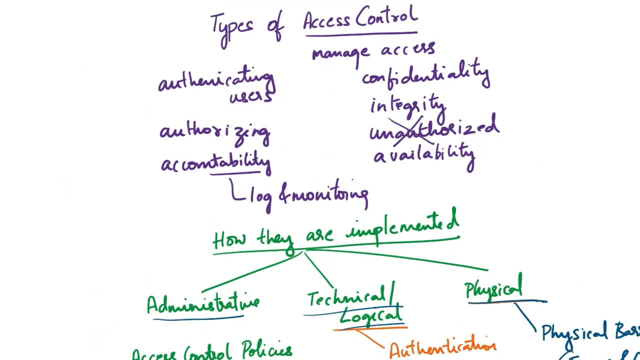 appropriate access to resources, systems and information, while preventing unauthorized access. it aims to strike a balance between enabling access for legitimate users and safeguarding sensitive data and resources from unauthorized disclosure, modification or misuse. that it is, that is, it is trying to identify and authenticate the data and resources that are available to the. 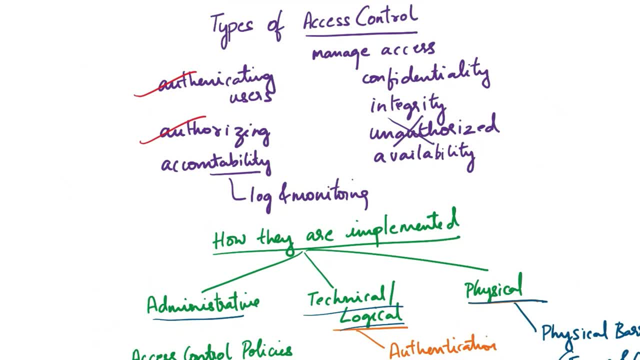 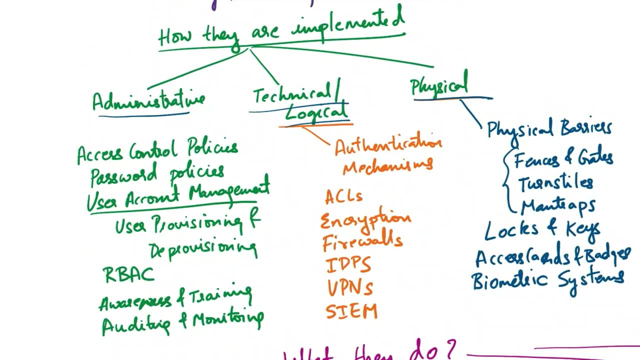 user so that it can be used to authenticate the user, authorize them based on their roles and permissions, and then also provide accountability by using logs and monitoring systems. then we have different types of access control. the first type is based on how they are implemented. administrative access control involves policies, procedures and managerial oversight to regulate user access and